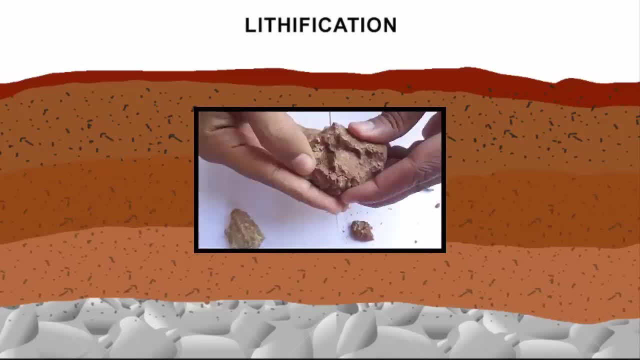 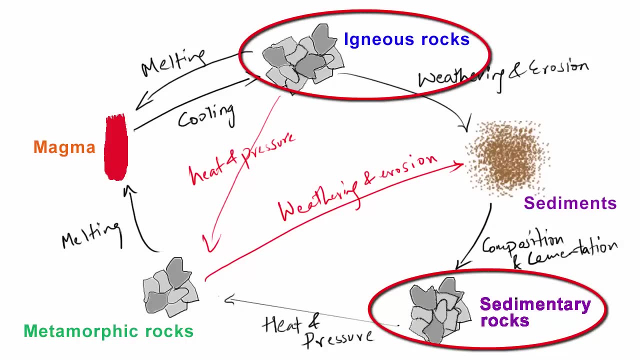 a sedimentary rock breaks into smaller chunks or debris, And when you see those debris you can easily relate what I'm talking about. So that was the formation of sedimentary rocks from igneous rocks. Now this sedimentary rock has the tendency to break apart again into smaller 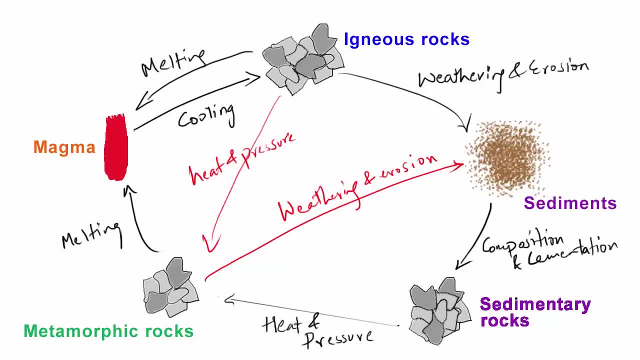 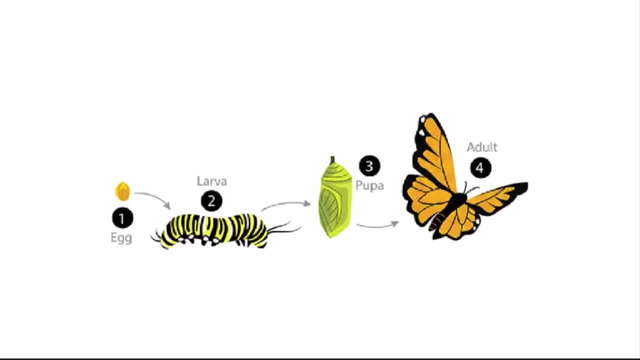 debris or sediments. Now comes the part where we need to find out how metamorphic rocks are formed. Do you remember that caterpillar changes into butterfly? We call that process as metamorphic. What are these metamorphic rocks? I will tell you, For example, there are some metamorphic rocks. 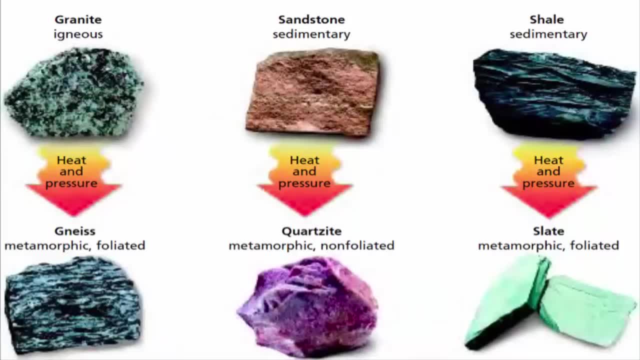 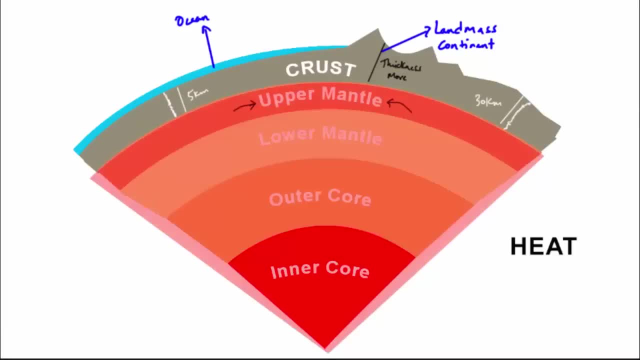 in our climate, called earth's tectonic plate, Which is basically pour Ziems And some of the maddening heat induced careful amounts of radiation inside to the Earth, which caused the earth to move further and further and the origination of ice cube'srá. 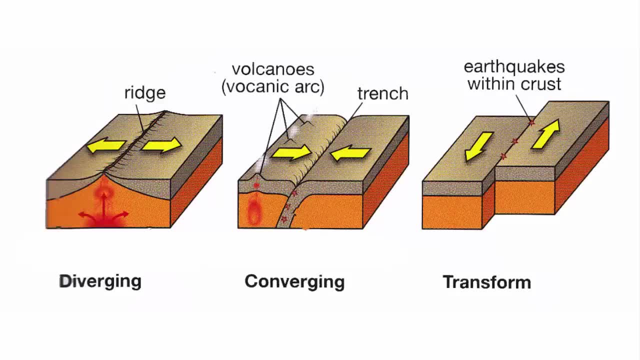 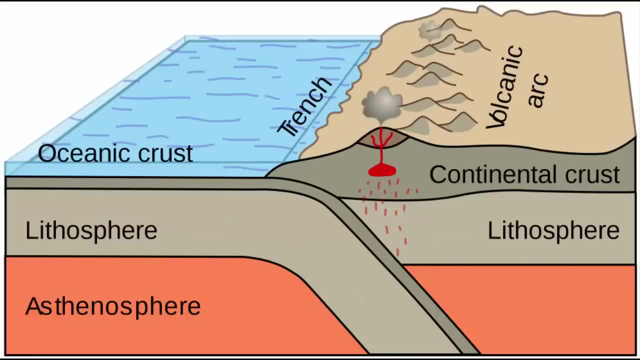 in the formation of concentrated crystalline minerals In ones CHRISTAL Period. there are bowels covering the earth, and they are called'túsvtet' orbutritatirchy'. So this metamorphicм occurs in rocks as well, especially when they are heated to 300-700ºS. 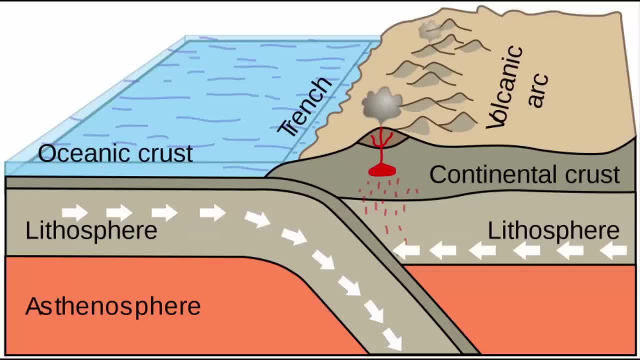 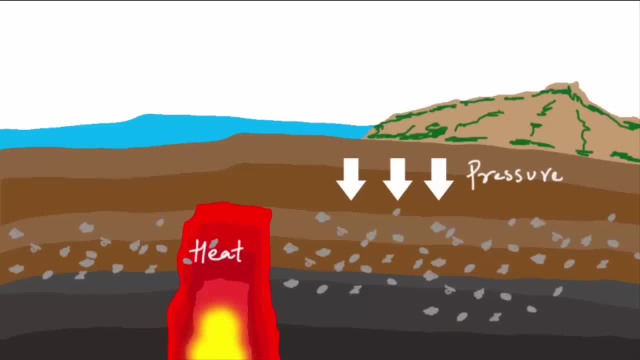 that is also a tremendous amount of pressure and heat. Now that we know how the heat comes from, what does this heat do to the rocks? It bakes them, Just like how you bake a cookie from dough. it does not melt the dough right, It changes its form. Similarly, rocks do not melt. 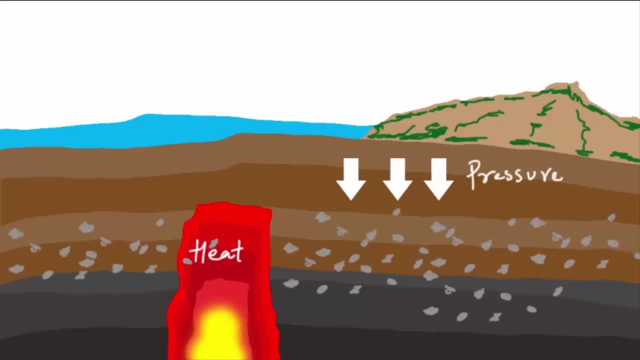 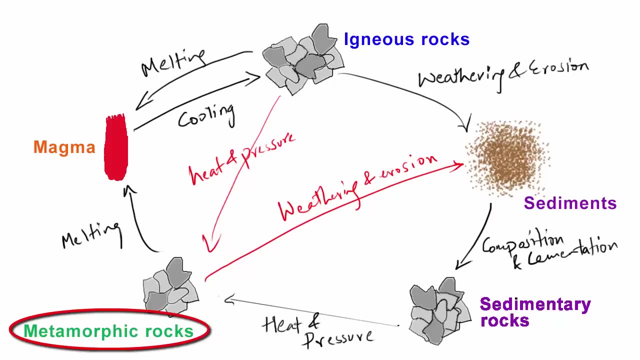 it transforms into metamorphic rocks. That's why you'll find metamorphic rocks mostly in mountain areas And, again with exogenous forces like wind, water, these metamorphic rocks can be broken and washed away into sediments, And these sediments can again make sedimentary rocks. 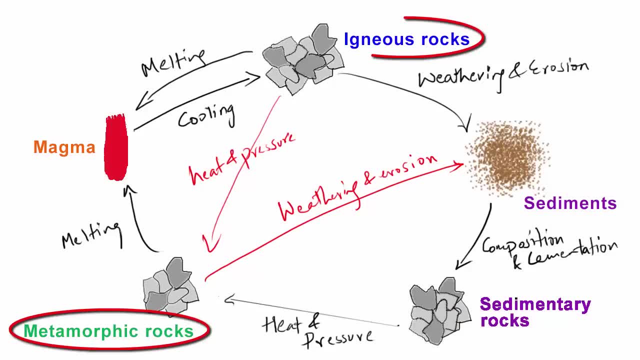 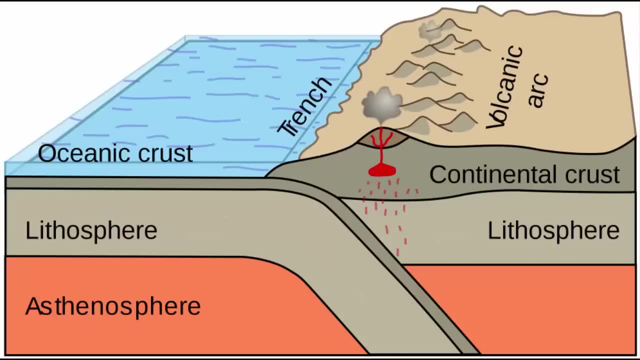 The rock cycle never stops. Metamorphic and igneous rocks find their way into the mantle through subduction. It happens when two plate converges and then one plate goes under another. This way, all these metamorphic and igneous rocks find their way into the mantle. 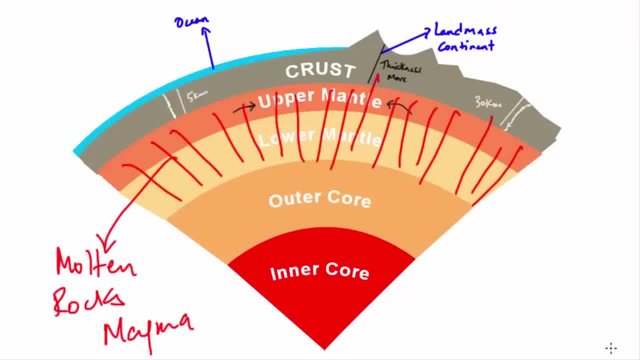 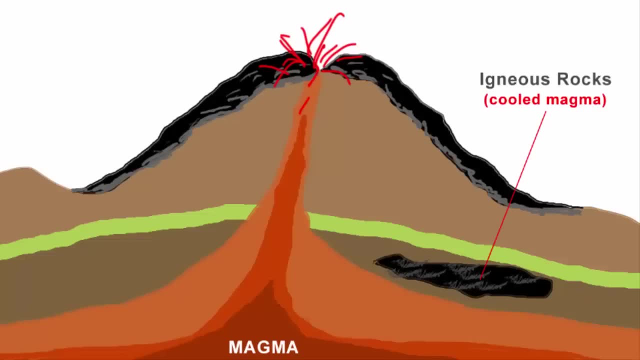 And we know mantle consists of molten rocks called magma. And again, magma comes out on the surface through volcanic activity And that's why we call it a metamorphic rock. That's how you find the sources of igneous rocks. So this is the rock cycle. I hope you understood. 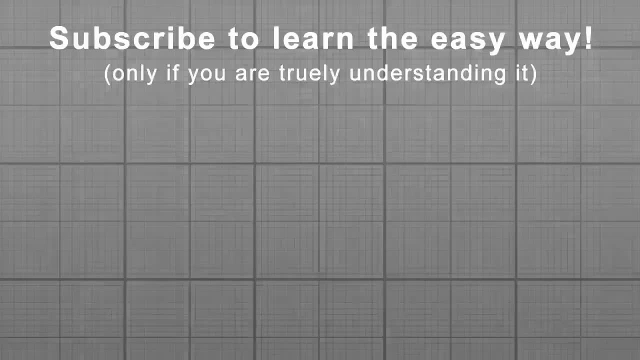 with this illustration. If you want to see more of such educational content, make sure you're subscribed. By doing so, you'll get an alert when my next video comes. Thanks for watching and I'll see you in the next one.